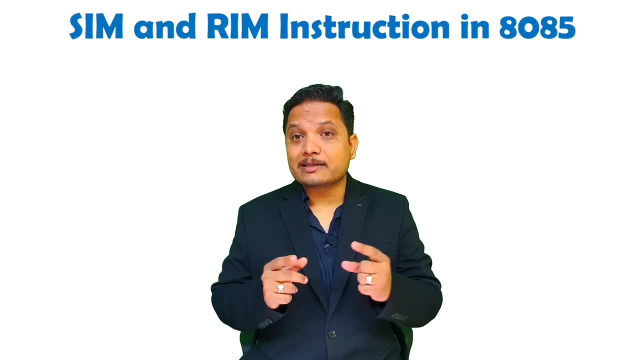 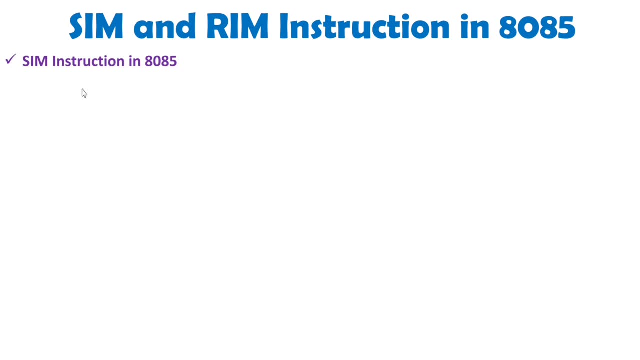 interrupt status. So how to have all those things? Let us try to understand that step by step. So, my dear students, first of all I'll be explaining you SIM instruction in 8085.. SIM means set interrupt mask. So here we are delivered: to set interrupt mask by using 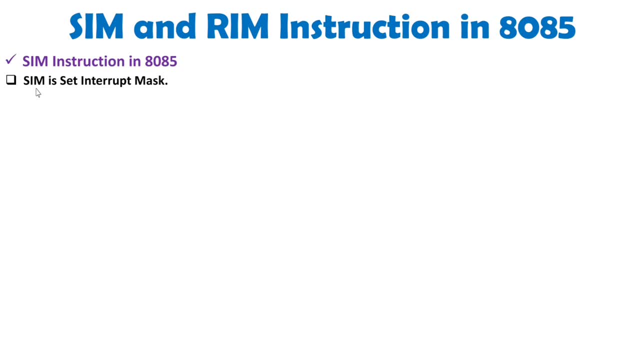 SIM instruction in which we need to see how command is there with SIM instruction and it is operated along with accumulator. So first of all you will have to load the value of accumulator. that will be your command. After that you will have to write SIM instruction. 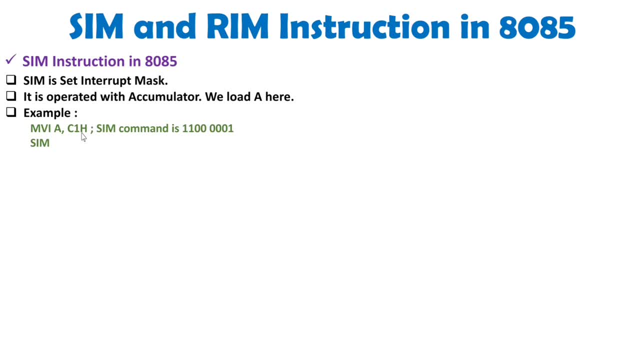 I've write MVIA, comma C1 hex. In that case you can say C1, that is getting loaded into accumulator, So that will be now command for SIM instruction. So after that, if you execute SIM, then this C1 hex, that is 11000001, that will be command which will be given as per SIM instruction. So let us see. 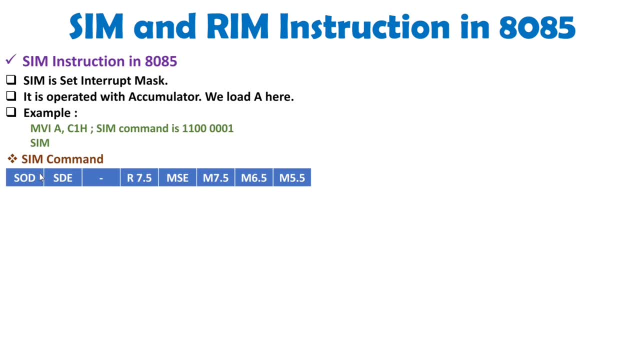 how this command is used to set interrupt status as well as context, because we don't want to send any emails or data in our system. So let us try to start with the video. So, my dear students, let me show you how the command works. Let us see how we can set up the command of SEM instruction. 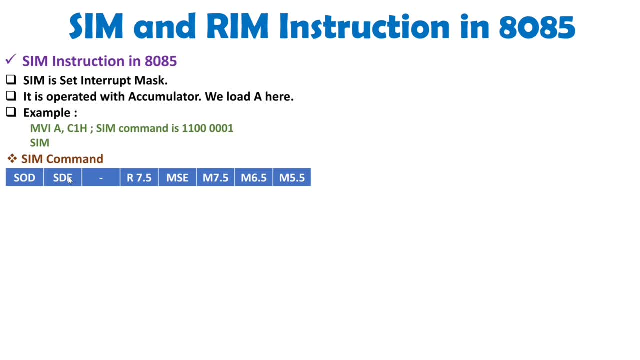 Let us start with SEM instruction. So, for example, we have already created a command. So, my dear students, this is the command with SIM instruction. So let us see how this command works. So, my dear, So if this is equals to 1, in that case we are enabling serial communication. 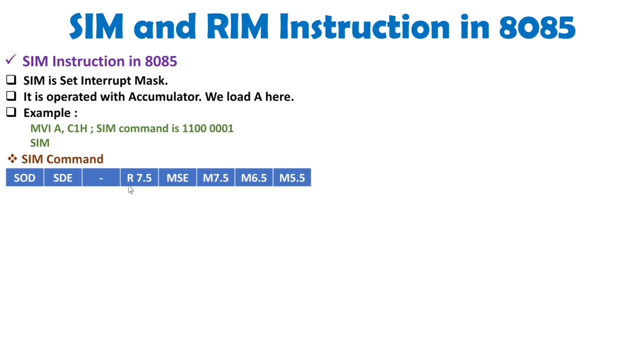 After that you can send 0 or 1 from here And this 5 bits- that is there to set up interrupt. where you see this: M7.5,, 6.5 and 5.5, that is to set mask of interrupt. 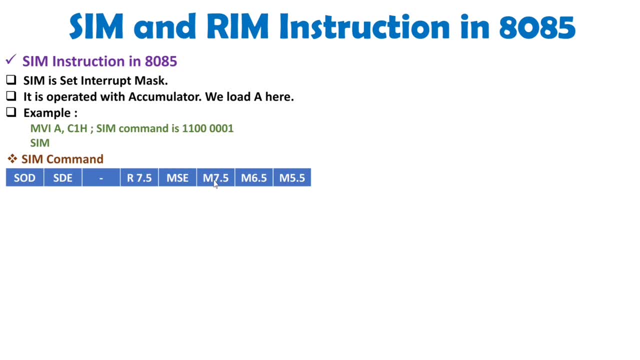 We have already seen hardware interrupt of 8085.. In that RST 7.5, 6.5 and 5.5, that were there that we can mask by using these 3 bits that even we have already seen in its structure of interrupt. 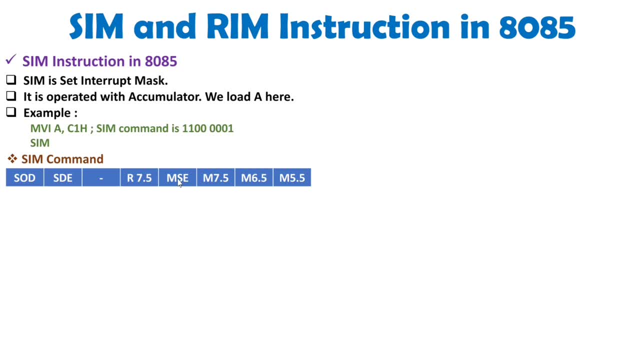 And to enable mask. this MSE bit is there And this R7.5 bit that is to reset, interrupt, RST 7.5.. So let us see all those bits step by step. So here, as I have told you this, 3.5.. 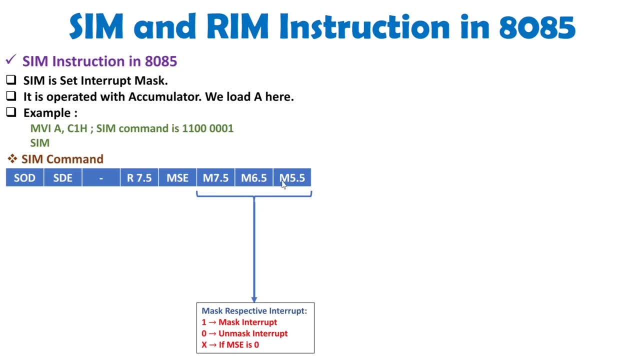 These 3 bits- M7.5, M6.5 and M5.5, that is to mask interrupt. So here, if it is 1,, then we are masking that interrupt, And if it is 0,, then we are not masking that interrupt. 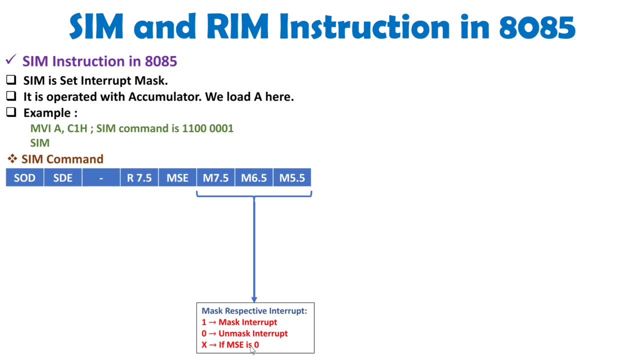 And that will be, don't care, as if MSE is equals to 0.. So first of all we need to set interrupt mask by this bit. So you will be observing if this bit is equals to 1. Then we are enabling mask. 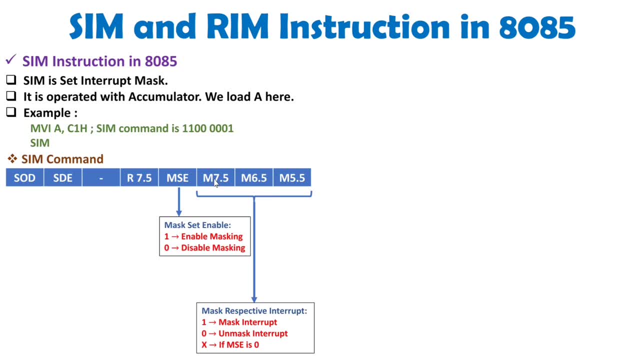 If it is equals to 0, in that case we cannot do anything with these 3 bits. Let us say you are having, this bit is equals to 1.. And let us say you are writing 001 over here. So what it means: here we are masking RST 5.5 hardware interrupt. 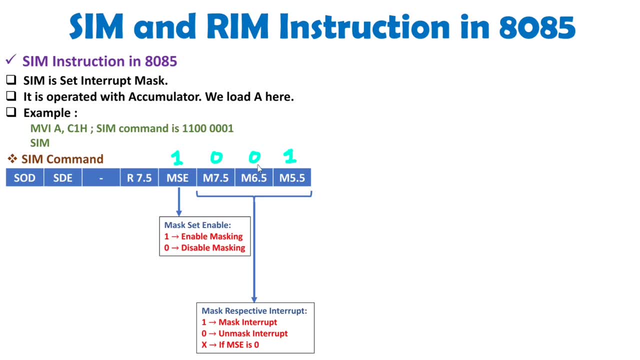 And if values are 0, then we are not masking that interrupt. But for that it is very complicated, Very compulsory- that you will have to make sure this MSE bit, that should be equals to 1. That will enable masking of these 3 bits. 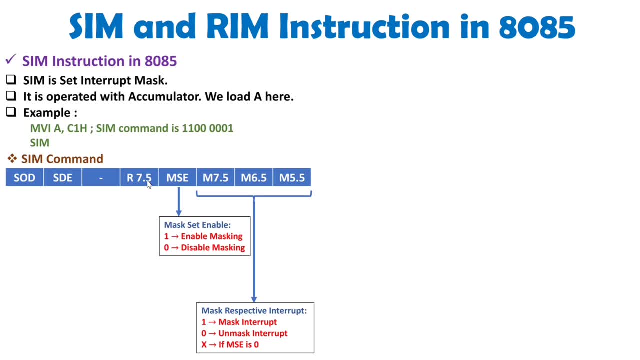 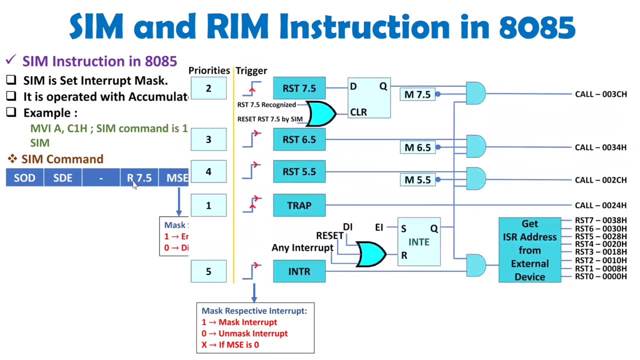 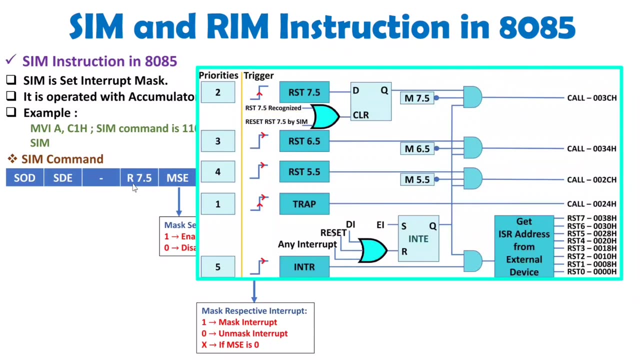 Now this R7.5, that is to reset RST 7.5 interrupt. If you see my video based on complete structure of interrupt, In that we have seen RST 7.5 interrupt is age trigger interrupt And RST 7.5 interrupt is age trigger interrupt. 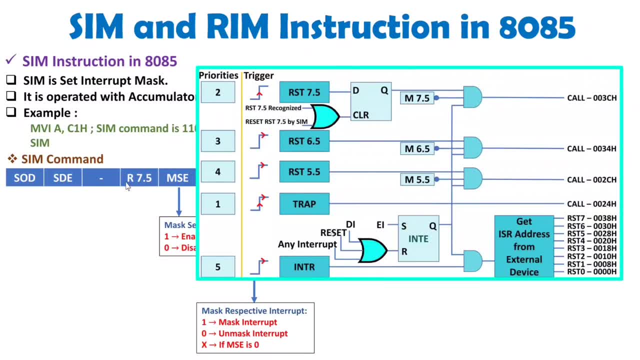 After generation of interrupt there was D flip-flop And clear terminal of that D flip-flop was connected with reset RST 7.5. And by having that reset we can clear that flip-flop. So if interrupt is pending, then also we can clear that flip-flop. 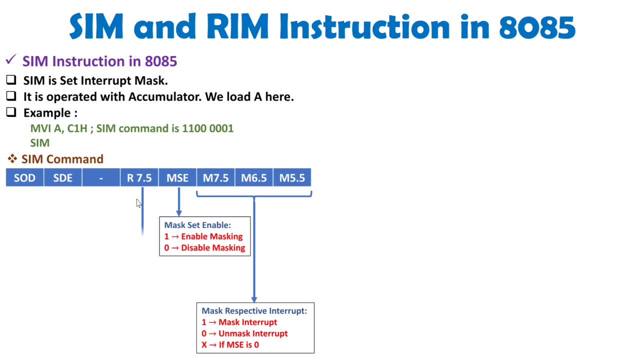 For that. that bit was connected there. So if this bit is equals to 1, then you can reset RST 7.5. And if it is 0, then we don't reset that. You can have execution of that interrupt as if it is pending. 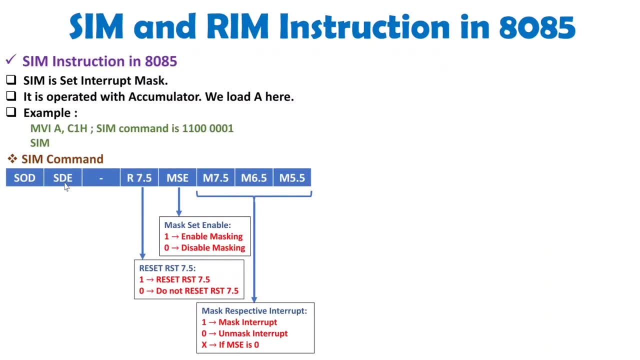 And, as I have explained, this SDE, that is, serial data enable. If it is equals to 1,, then we are enabling serial data communication, And if it is equals to 0,, then we are disabling that serial data communication. And if this bit is equals to 1,, then we are disabling that serial data communication. 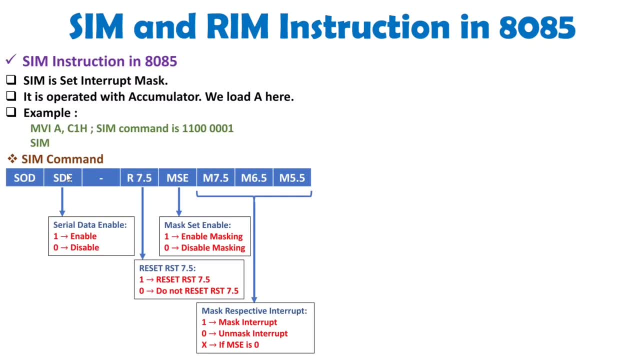 And if this bit is equals to 1,, then that is enabled. In that case, here we can transmit that 0 or 1.. If it is equals to 0,, in that case we transmit 0 over here, provided 1 is over here. 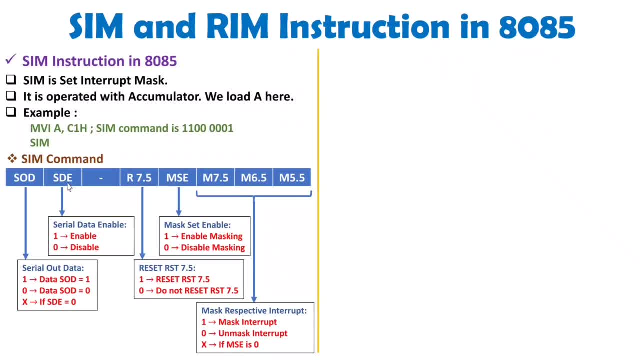 And if it is having 1 over here, provided 1 over here. in that case, we are transmitting 1 serially And this will be, don't care, as if this bit is equals to 0.. So, my dear students, this is all about SIM command, which explains you two things. 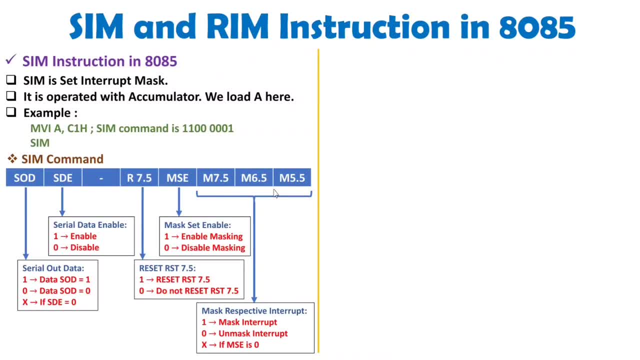 One is serial communication and second is set interrupt mask. Now I will be going to explain you what will happen with RIM instruction in 8085.. RIM is read interrupt mask. So here we will be reading interrupt mask And that is also operating along with accumulator. 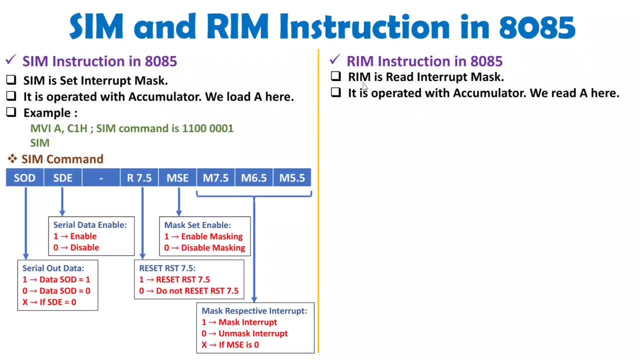 When you write RIM is instruction RIM, at that time you will have to see what is the data which is there with accumulator And whatever data that is there with accumulator that is been showing status of RIM command. So, for example, here if I write RIM and after that if you have, accumulator is equals to 8, 8, hex. 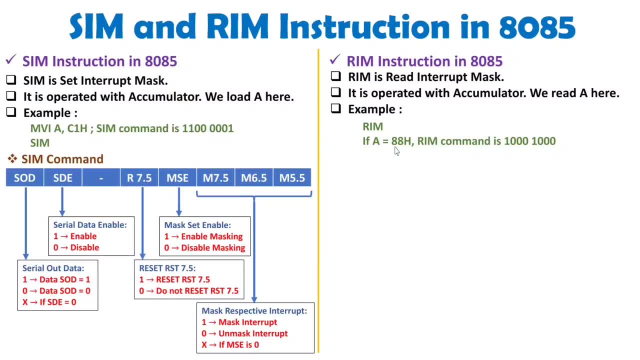 it means RIM command, that is 8, 8. hex means 1 3 0 0. 1 3 0 0.. Let us see what is that RIM command. So RIM command also explains you status of interrupt as well, as here we can have serial in data communication. 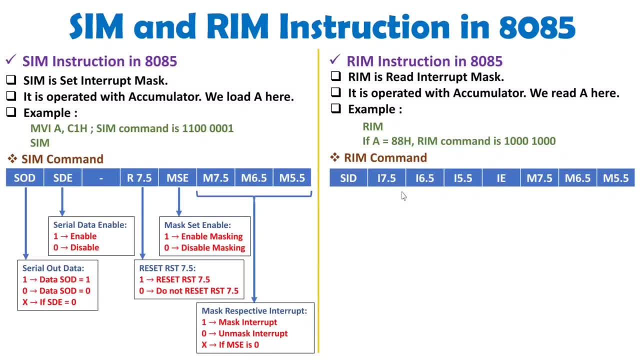 So here see this 7 bits that is showing you status of interrupt and this 1 bit that is been showing you what serial data that we receive. So here how status is been read. Let us try to understand that So as if you see this 3 bits. 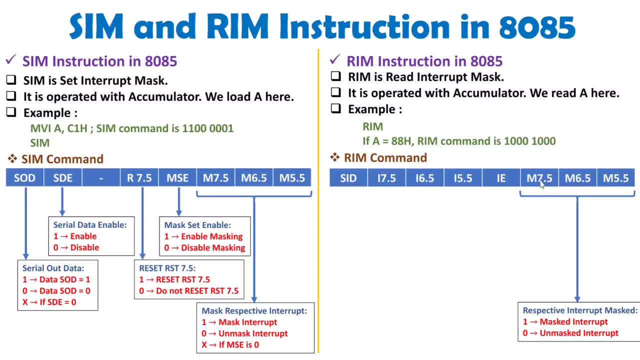 So if this bits are masked, in that case it will be 1.. So here we can mask the bit. But if it is showing this bits are 1, in that case you can say: respected hardware. RST 7.5, RST 6.5, RST 5.5 interrupts were masked over here. 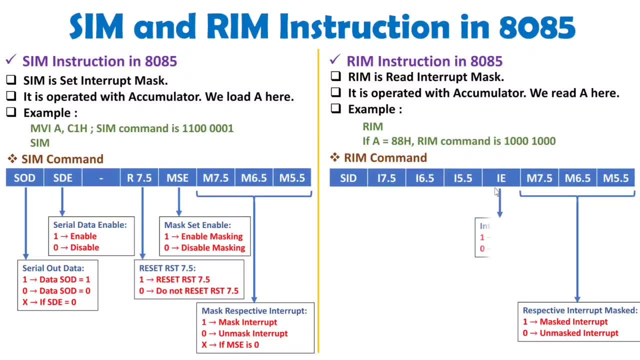 This IE that explains you interrupt enable. If it is equal To 1,, then you can say: interrupt is enabled, and if it is equals to 0, then interrupt is disabled. If it is equals to 0, interrupt is disabled. What it means: no more interrupt can be recognized as if it is generated other than trap interrupt. 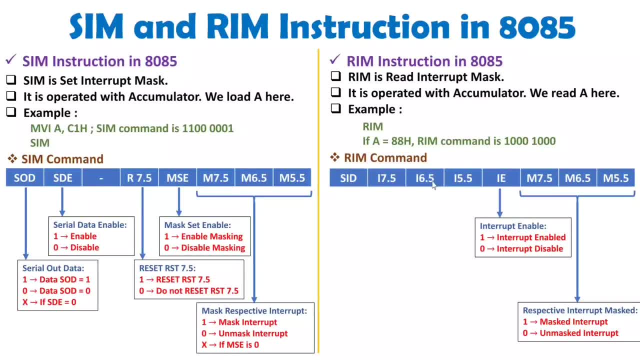 Now this 3 bits: I 7.5,, I 6.5,, I 5.5. that explains you pending status of interrupt. So if any interrupt is pending, Then it will be indicated by 1 over here and if you will be having 0 over here, you can say respective interrupt is not pending and, as I have told you, this is therefore serial in data. so that will be indicating what data that we have received. if it is equals to 1, you can say we have received 1 over here and if it is equals to 0, you can say we have received 0 over here. 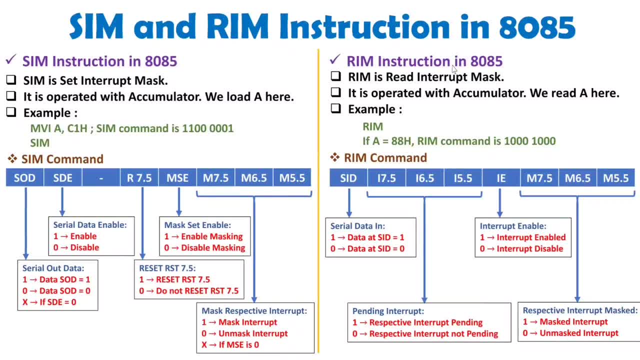 So, my dear students, Sim and Ream, that is having two operations. One is for serial communication. Here, by having sim we can transmit serial data and by having Ream we can read serial input data to microprocessor. By having sim we can set interrupt commands and by having Ream we can read the status of interrupt right now. 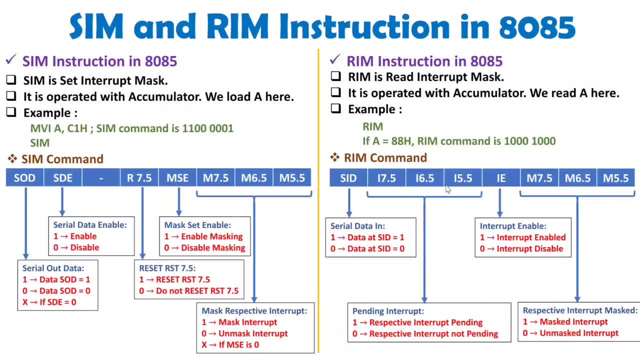 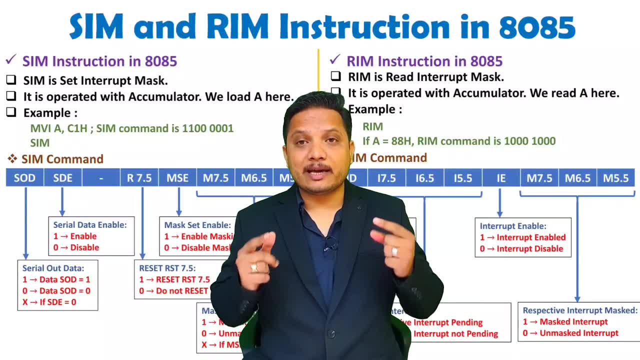 So that is how these two instructions are there, and these two instructions are very essential. And these two instructions, My dear students, I'll be making two separate videos for different case of Programming. one video that I'll make it to generate one square wave by using sim instruction.